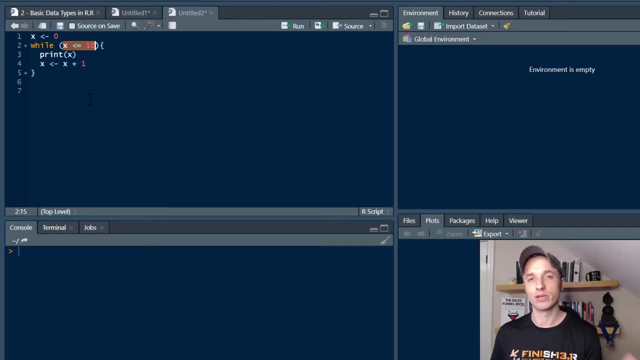 So it's gonna run for a set number of times and we'll go through that together during this video here. So anyway, let me go ahead and run this loop real quick so we can see what it produces. So it produces a list of numbers 0 through 10, right? 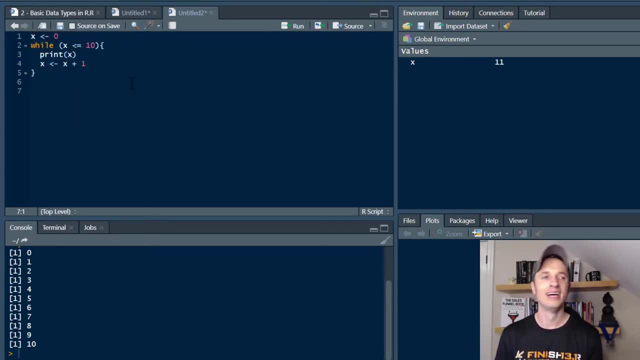 So that's, that's what the loop does. and now let's go ahead and make it for loop that does the same thing. So, to do it, We type out 4, and then we go ahead and throw in our parentheses here, and then we go ahead and set a variable. 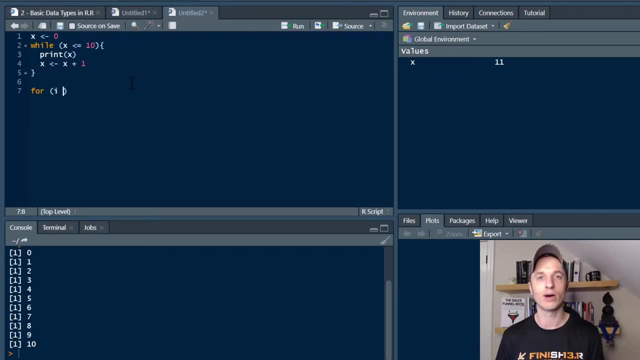 I is like a default variable, but you could put whatever you want in there. You can put a word in there if you want to. it doesn't matter this. the same concept will apply. So we got I in is the next piece of language, the next piece of code that you want to go ahead and use, and then you usually give it a range and 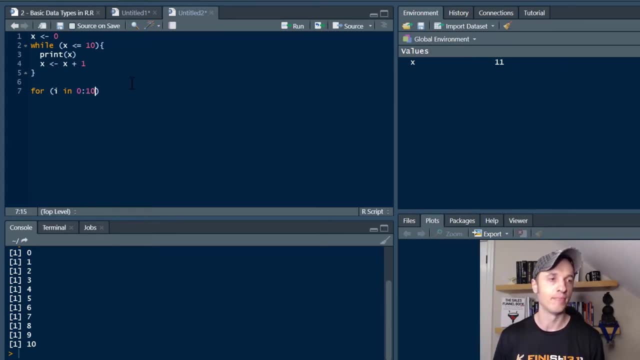 In this case, I want to go ahead and give it 0 through 10. now, this right here is what we call a vector, and you can do several different things with vectors, and I'll have another video on vectors because They're pretty flexible, but you think of it like an array. 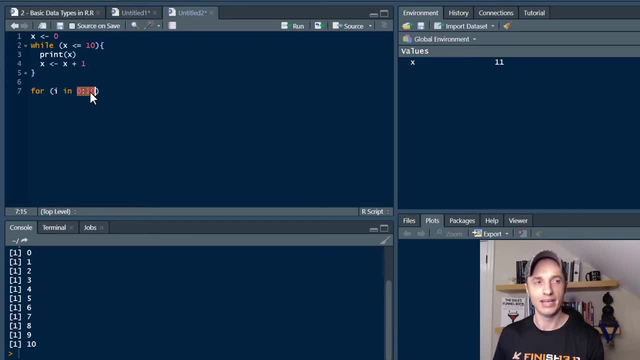 So it's, like you know, a list of numbers 0 through 10, essentially right here. So if I highlight this and I can run it real quick When you show, when you see what it looks like, so you see it, just you know list out basically 0 through 10. 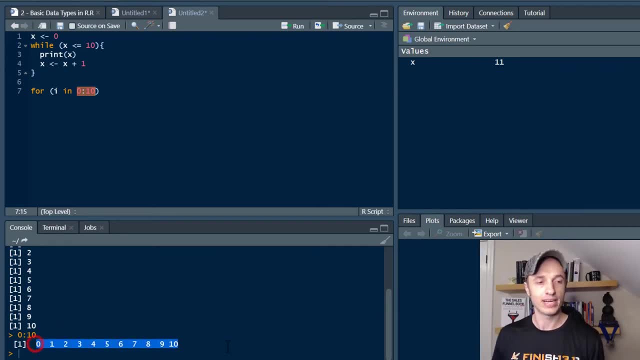 so that's an array of Numbers or a vector from 0 through 10.. So there's basically the point is, there's essentially Well 11 items in this vector right: 1, 2, 3, 4, 5, 6, 7, 8, 9, 10, 11, right. 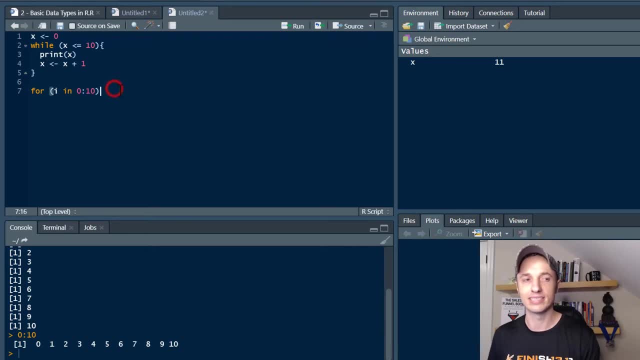 So 11 items in that vector is essentially what this is saying here. So next up, we'll go ahead and throw in our brackets or squirrely brackets and we'll go ahead and print and I Okay. so let's go ahead and run this loop real quick. 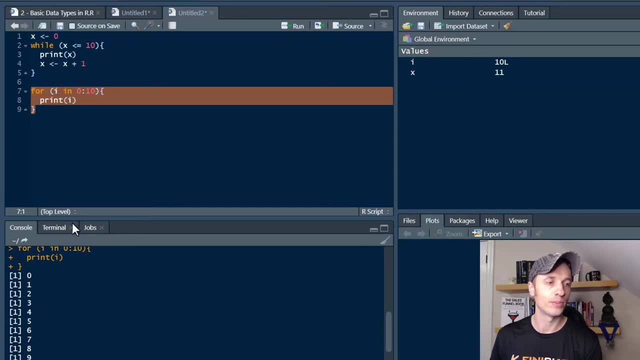 And we see we get the same result as the while loop up here. We get 0, 3, 10 printed out and you notice that you know that's two lines shorter and simpler than the while loop. So that's why you'll typically use a for loop when you're you're iterating a set number of times, because you know. 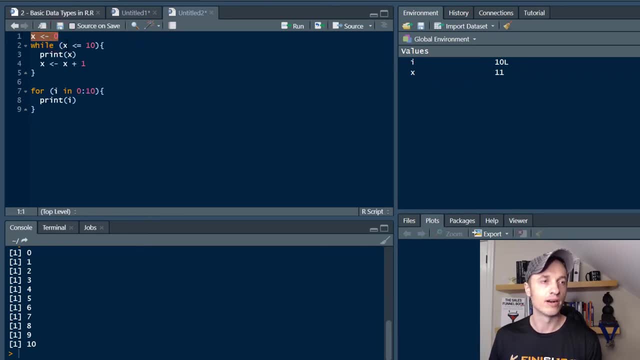 it's a cleaner way to do it. then you know setting a variable to 0, and then less than or equal to, and then you Got to add and you know count up until you reach whatever number. So for loops are great for counting through a set number of times and now your vector can be, you know, any range. 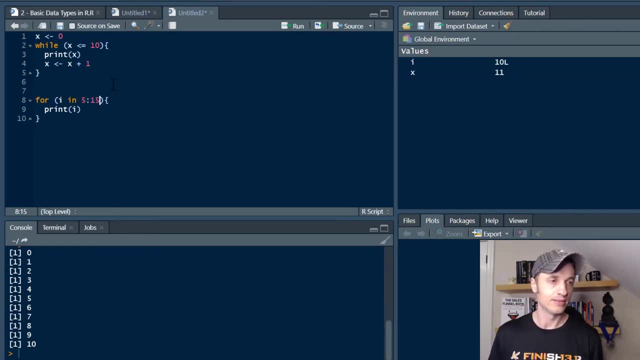 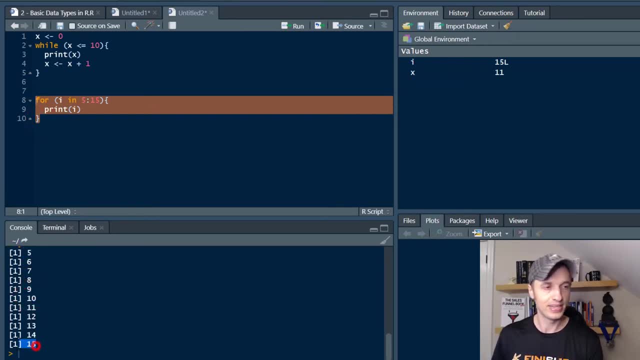 What it prints out. so we get you know 5 through 15 printed out instead of 0 through 10, right? Alternatively, what we could go ahead and do is if we just run it by, like we want to print high, and let me just make this 10 times so we can. 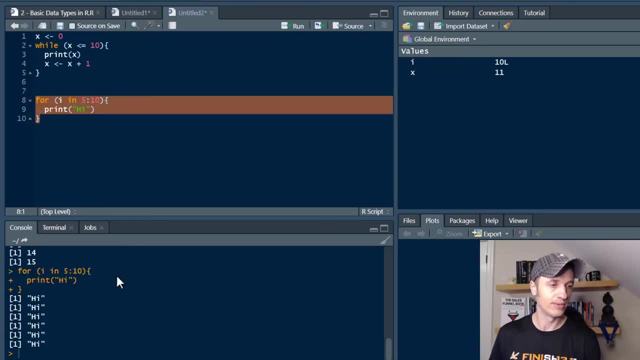 We have less to look at. so if I run this real quick, we see that it prints out high 1, 2, 3, 4, 5, 6 times right. so you know 5, 6, 7, 8, 9, 10, you know. 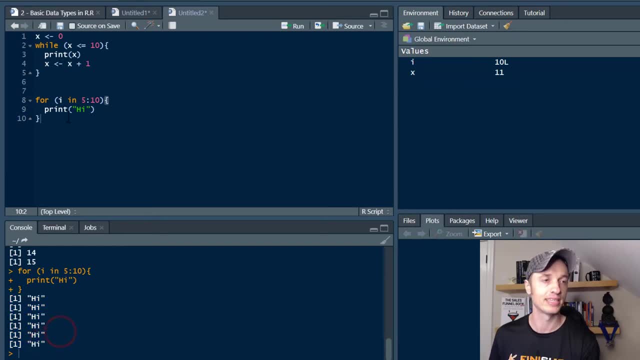 That's 6 times, and so I print it out high 6 times. So, basically, it runs through the loop, However, however many items are in this vector. So that's something important right there. I'm going to say it again: It runs through the for loop runs through however many items are in a vector. now, 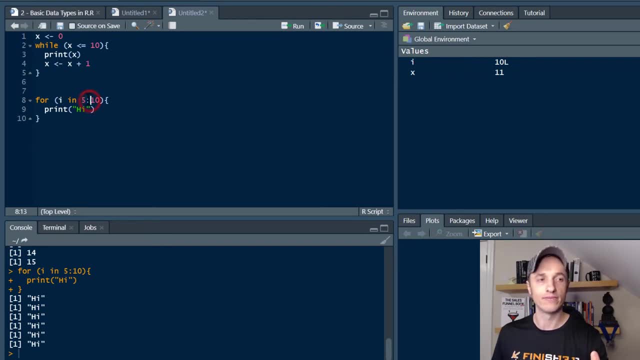 This is a way to set up a vector- is with the colon here, So 5, colon 10 as a way to set up a vector, but another way, And this is just a quick overview of vectors. again, I'll have another video on vectors. So because there's more to them then what I'm showing you here 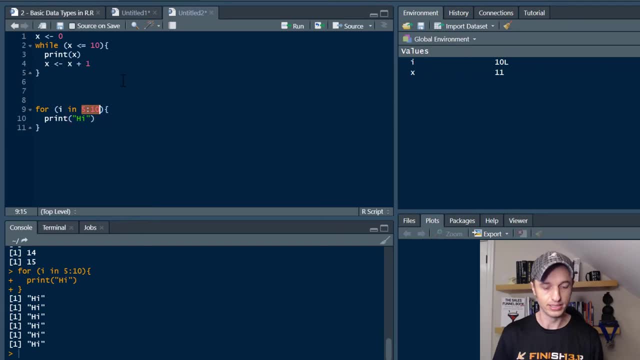 but another way you could go ahead and do a vector is use a C for combined and then use the Parentheses and then we can throw in numbers or items here. so just for a safe example, do 0, 1, 2, 3, 4, 5 and. 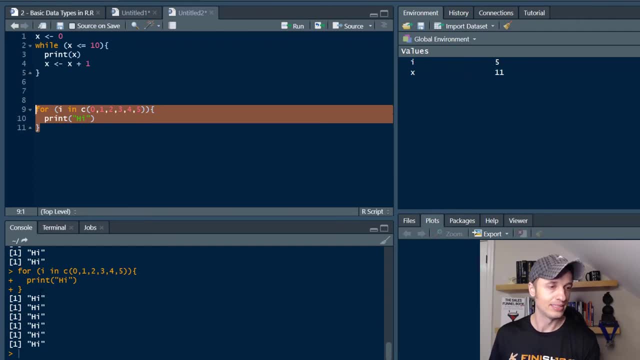 I'll go ahead and highlight it and I'll go ahead and run it and we see we get high printed six times, just like we Had high printed six times up here. It just we, we did our vector, We like manually typed out our vector here. We put, you know, six items in our vector.